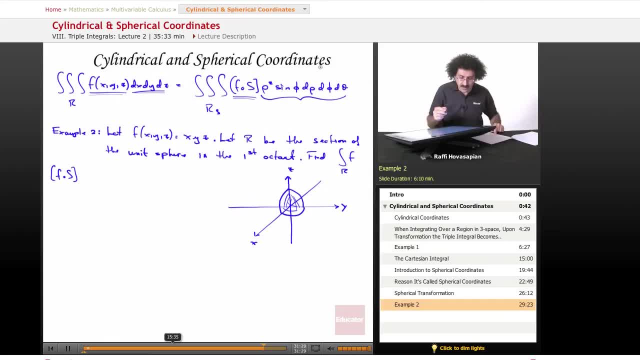 So f of s, so we can put it into our integral formula here. So f of s. well, f is x, y, z. x is r sine phi cosine theta. y is r sine phi sine theta. z is rho cosine phi. 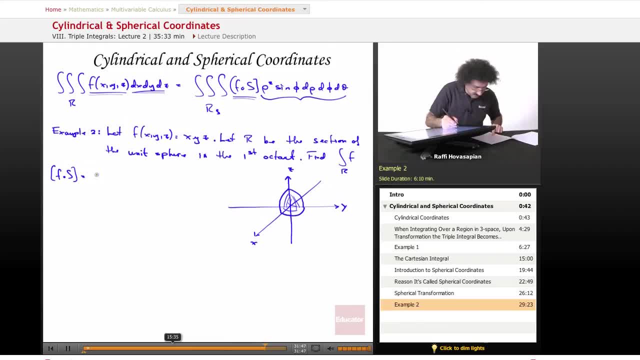 So we just put them in and multiply them out. So x, y, z is equal to rho sine phi cosine theta times rho sine phi sine theta times rho cosine phi. And I end up with- I want to simplify as much as possible. so rho cubed sine. 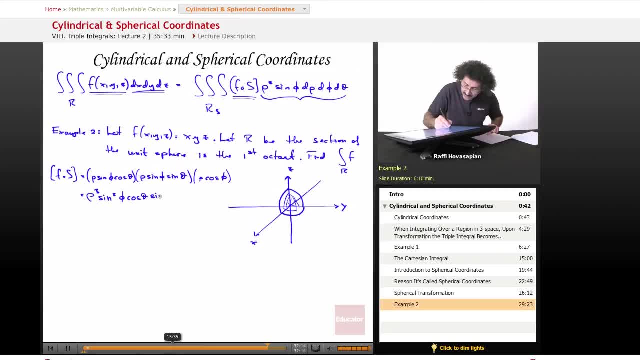 squared phi cosine, theta sine, theta cosine phi. OK, looks complicated, but it's easily handleable. Now we'll go ahead and do the integral. Well, let's see. First of all, let's go ahead and talk about so rho, let's see. 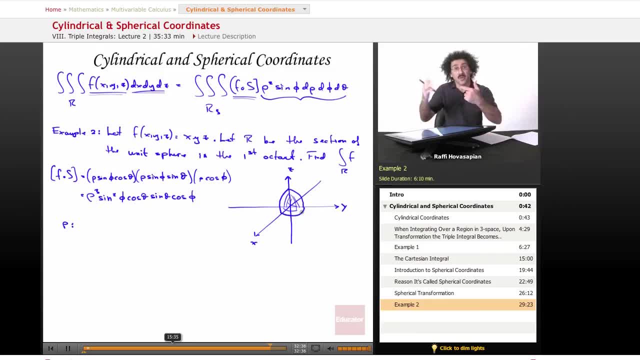 this is the unit sphere, So rho is going to go from 0 to 1.. 0 to 1.. Phi- well, phi is it's in the first octant, So it's going to be from 0 to pi over 2.. 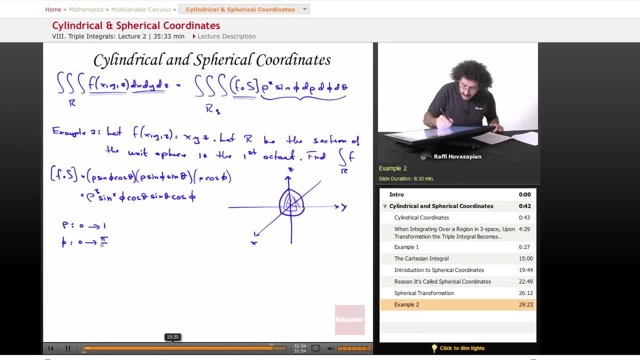 It's going to swing down through pi over 2, 90 degrees And theta is going to go from 0, again to pi over 2.. So 0 to pi over 2.. So now we're ready for our integral. 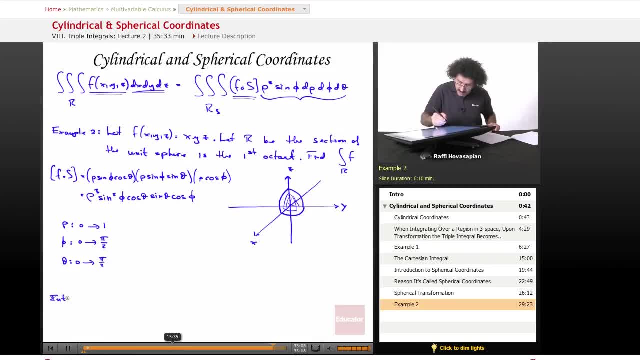 Our integral equals. that's OK, I'll go ahead and do it there. Integral Equals, So 0 to 1.. That's going to be our rho. We have 0 to pi over 2.. Let's make that our phi. 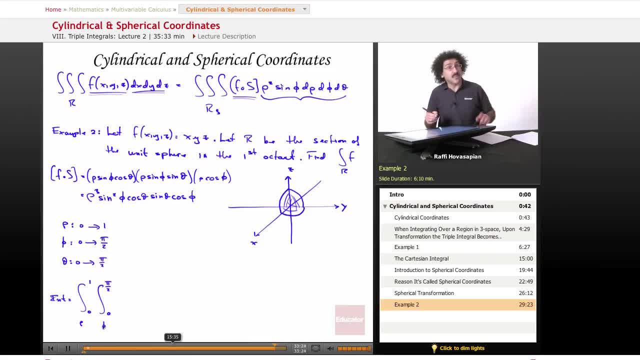 So I'll go ahead and write rho and phi- It's always good to write the variables underneath- And then our theta is going to be 0, again to pi over 2. And of course we have our function. So we have rho cubed sine squared phi. 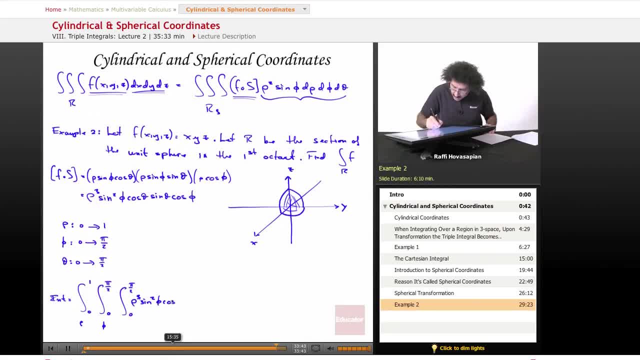 Just got to go slow. Make sure that everything is there, Cosine, theta. And again, be very careful with these, particularly because you're dealing with two angles, phi and theta. Don't confuse them, which I do all the time.